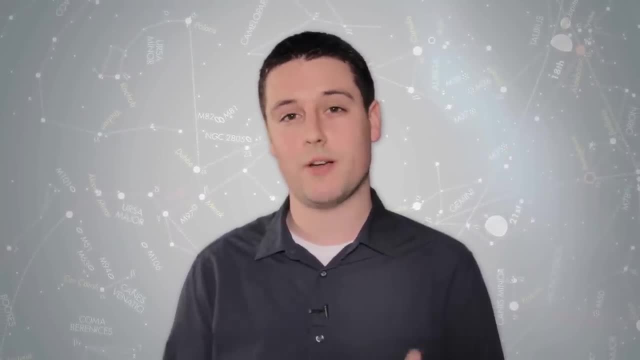 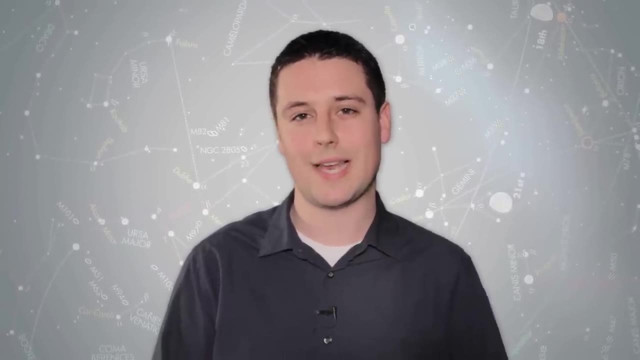 do want to take things further. you can pick up a pair of binoculars. A good pair of ten by fifty binoculars will allow you to see some of those star clusters in more detail and see more nebulae and more faint galaxies. 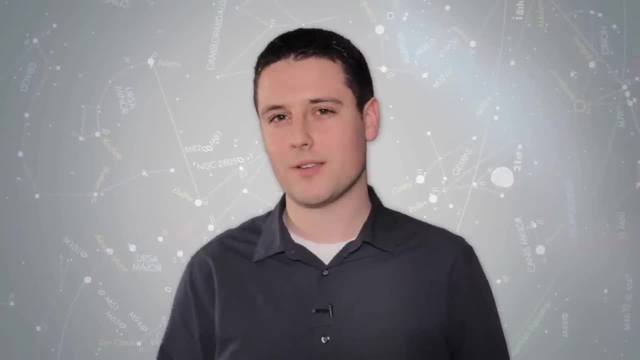 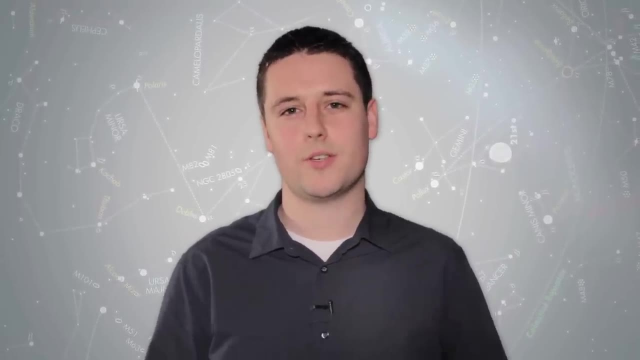 Tip number two is a very simple one, and that's to wrap up warm. Now, I know that sounds obvious, but actually a lot of astronomy is spent just standing still staring up at the sky, So it's really important that you insulate yourself from the cold. 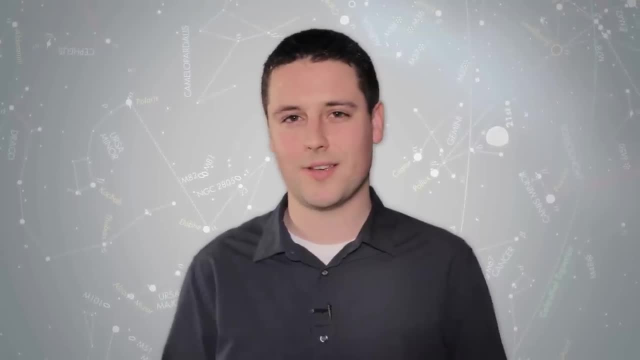 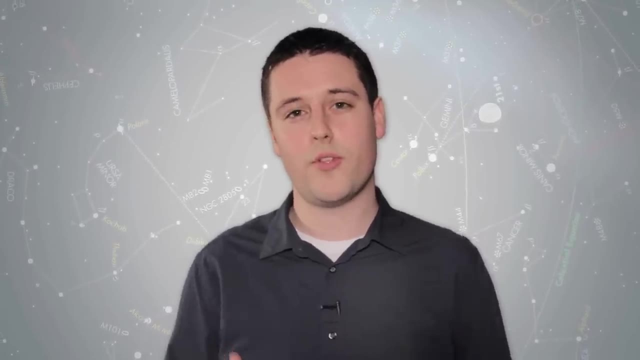 The last thing you want is to get out into beautiful, crisp, clear skies and then have to go indoors because you're too cold. So I wear a pair of waterproof shoes and waterproof trousers, as well as full thermals and a thick, warm coat. You need to insulate yourself against 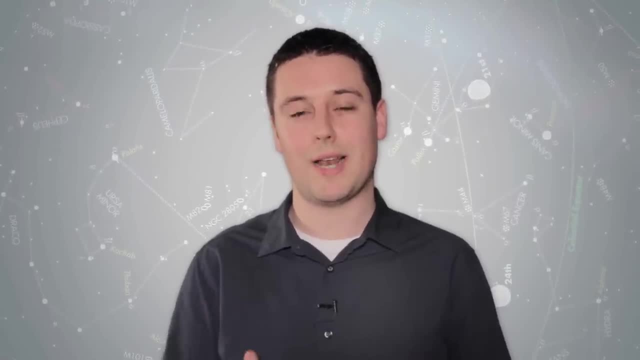 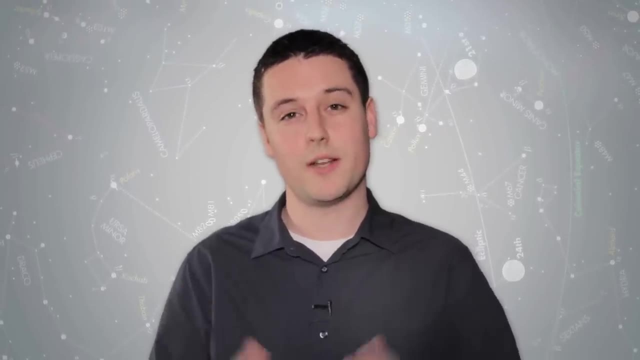 the cold, so lots of layers is a good idea. Also, I use a balaclava and hat to keep the chill off my face, and if you're using binoculars or a telescope or a star chart, a pair of fingerless gloves are a great idea. 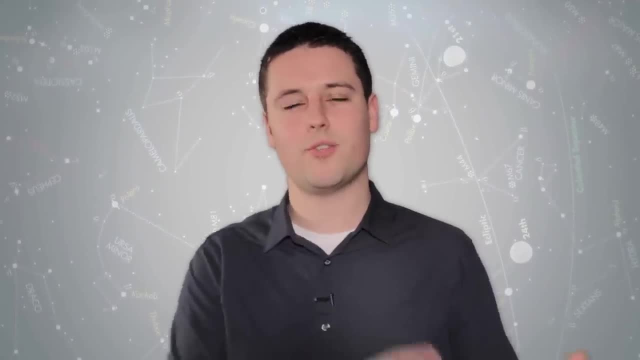 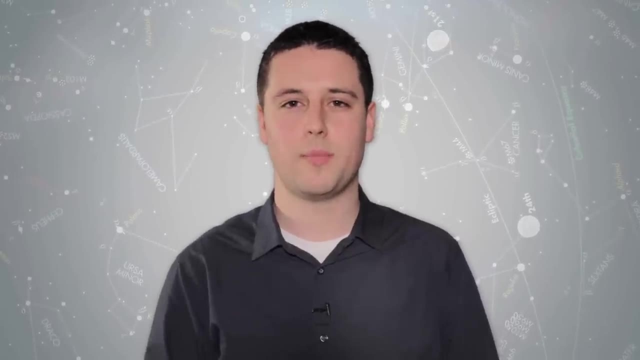 Tip number three: avoid street lights or any form of artificial light. really, If you can get out to the countryside, brilliant, because then you'll be able to take advantage of the dark skies there. There are lots of places in the UK where there are dark skies. 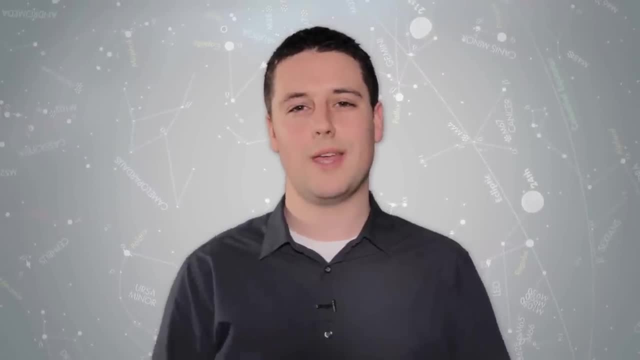 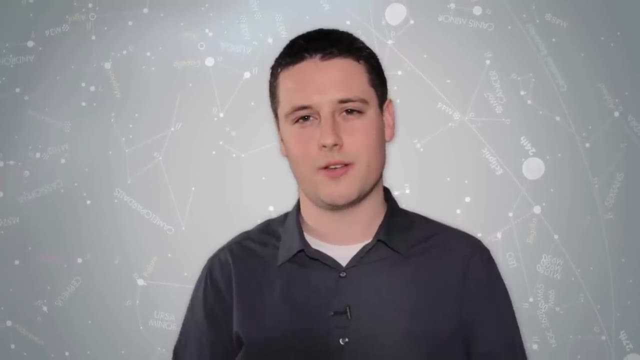 and that will really make a difference to your observing, because you'll be able to see a lot more, including things like the Milky Way and some of those faint galaxies I spoke about. My next tip is to let your eyes adjust to the darkness. Now. this is really crucial because 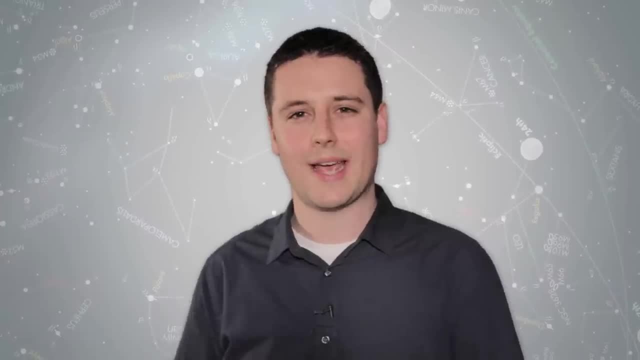 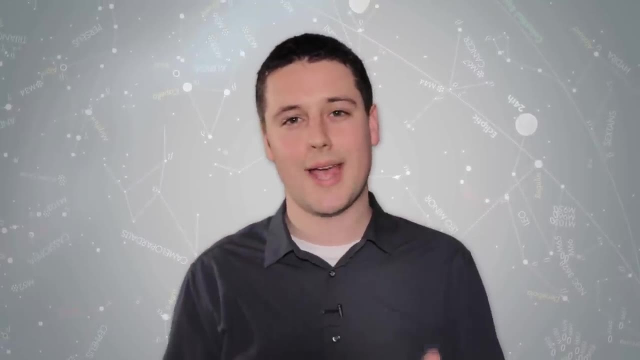 if you go outside from a brightly lit room or a brightly lit house, you'll probably only see a handful of stars. But if you go outside and then let your eyes adjust to the darkness for maybe half an hour to an hour, you'll notice an incredible difference. 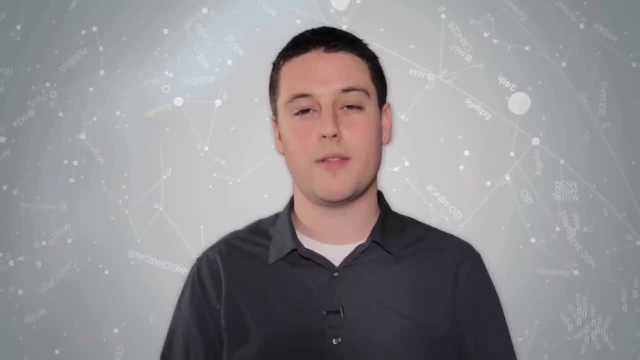 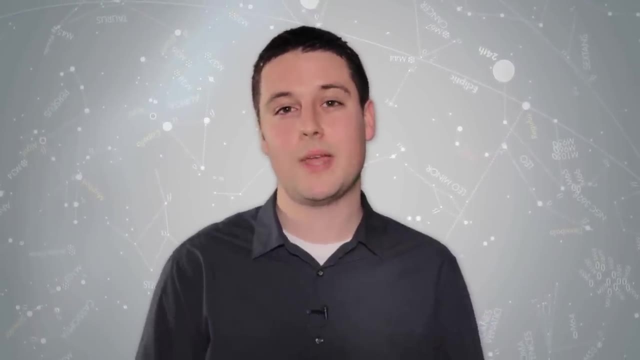 You should be able to spot many, many more faint stars and perhaps things like the Milky Way, from a site with very dark skies. Now my fifth and final tip is to pick up a star chart. Now we print one of these in Skartnight. 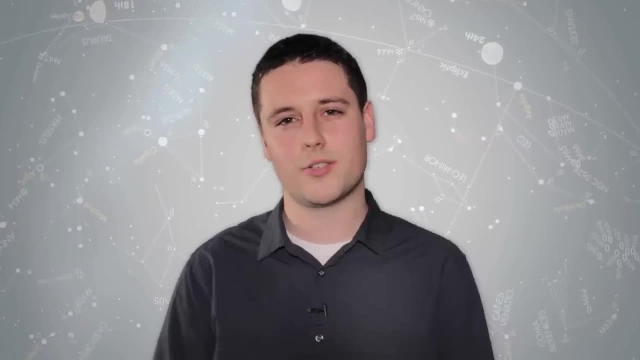 magazine every month, and they're a great way to learn your way around the night sky. You can begin by identifying patterns of bright stars and then go on to the constellation. I'm going to show you how to do that in just a few minutes. I'm going to show you how to do that in just a few minutes Now. my fifth and final tip is to pick up a star chart and we print one of these in Skartnight magazine every month and maybe even go on to the constellation. 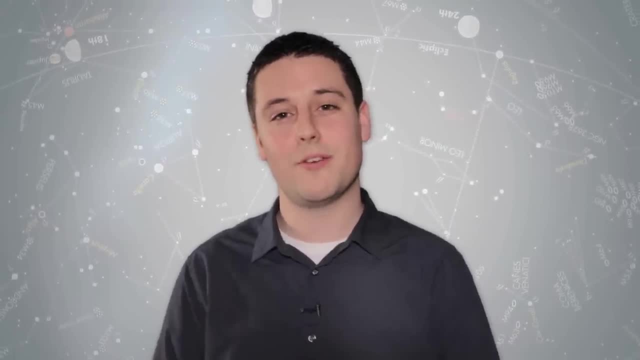 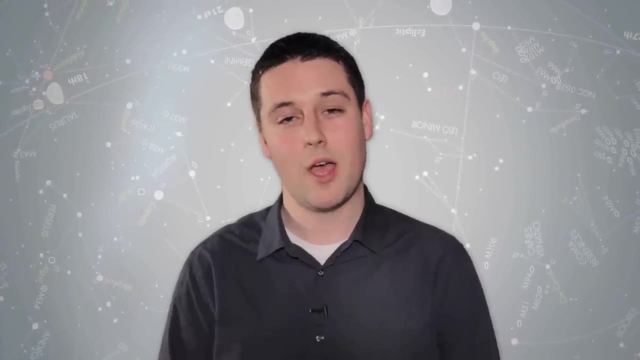 Now my fifth and final tip is to pick up a star chart and then go on to the constellation And before too long they'll become familiar and you'll easily be able to navigate your way around the night sky. So those are my five very simple tips for getting started in stargazing. I hope you.